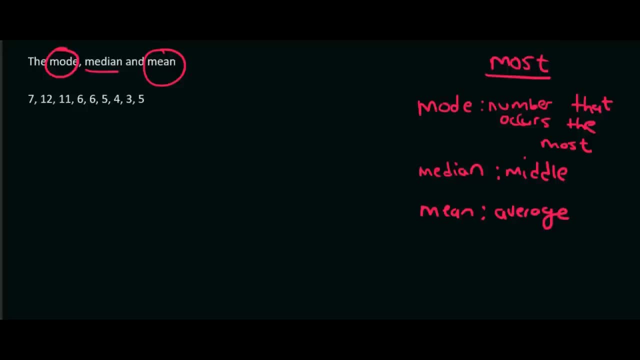 works in this video. But those are the three things you need to remember. The mode, it's the number that occurs the most. The median, it's the number that occurs the most. And then the median think of small, medium, large. So median is the middle one And then mean: well, that's when 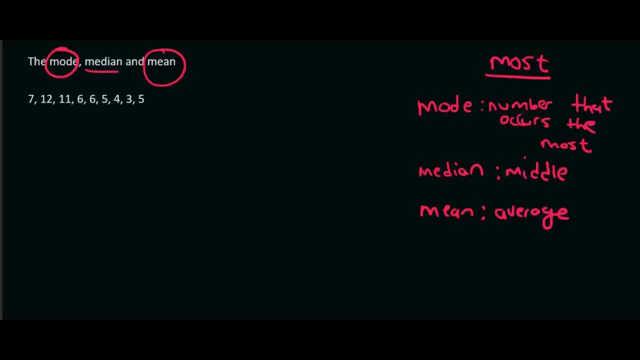 the teachers are being very mean because they're wasting your time. because you got to calculate that big, you got to do that big calculation And it's also just the average, Very, very important. I'm going to say that again. This is important. You must rearrange the numbers that they give you. 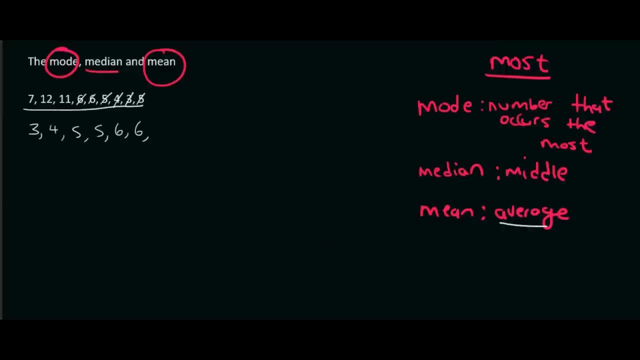 from smallest to biggest, And when doing so, please, in the test, just cross out the numbers that you have, And then you're going to have to do the same thing over and over again. Then another thing to do is to add up or to count these numbers as 1, 2,, 3,, 4,, 5,, 6,, 7,, 8,. 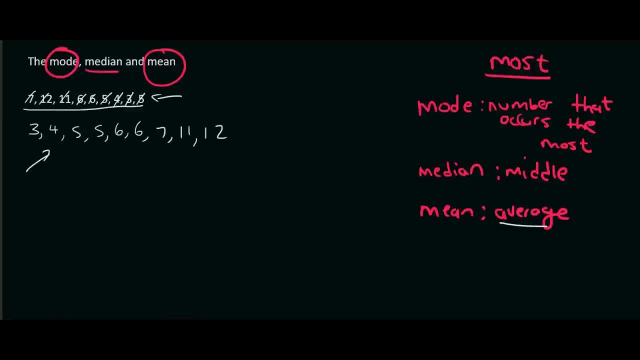 9 over here, And so we should have 9 over here. So that's 1,, 2,, 3,, 4,, 5,, 6,, 7,, 8,, 9.. So the chances are we've got everything, So let's find the mode. Well, we know that the mode is the number, that 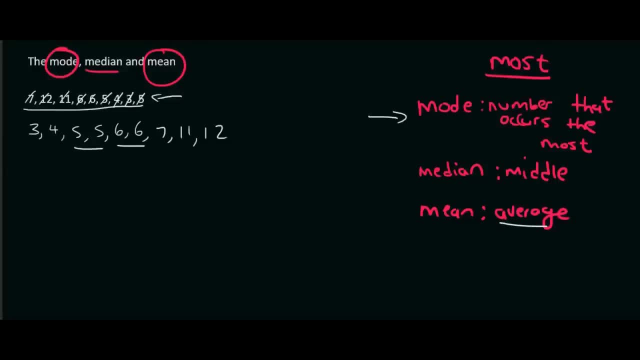 occurs the most. Well, there's two fives and there's two sixes, So unfortunately, for this one there is no mode. You can't have two modes, Okay, But if the five, if there was a third five, then our mode would be five And then median, or median is the number. that is exactly. 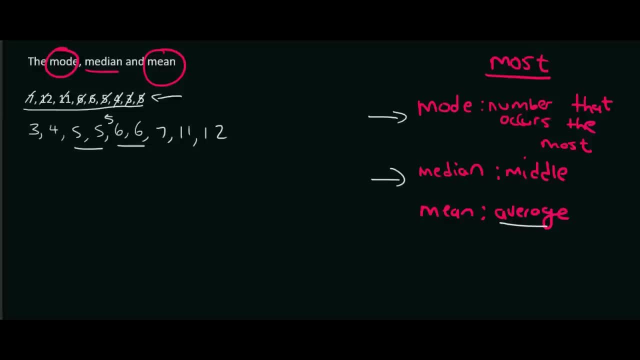 halfway Now. I've seen many ways to do this. One of the ways that grade tens like to use is this method. So you cross out there, you cross out there, you cross out there, there, there, there, there, there. That five wasn't actually part of it. And look what we left with right in the middle. 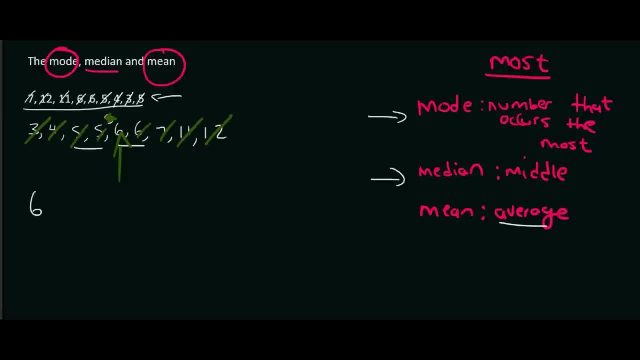 the number six, So the median would be the number six. Kevin, is there a more mathematical way to do this? Yes, The proper way to do it is to use the number six, So the median would be the number N plus one over two. Now this N is the number of items that we have. So we had nine items, That's. 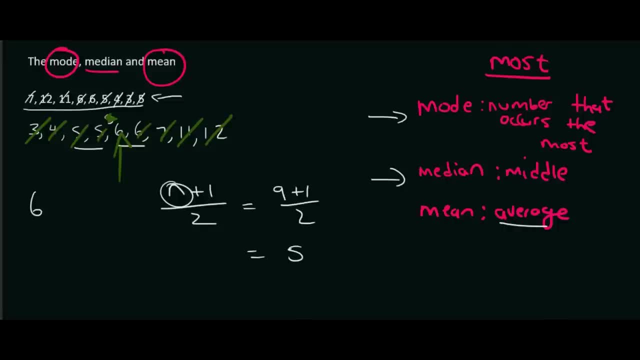 nine plus one over two, 10 divided by two is five. Kevin, I thought the answer was six. This is not the answer. That formula tells you the position of the answer, So we go to the position number five and that'll be one, two, three, four, five. Aha, So position five.